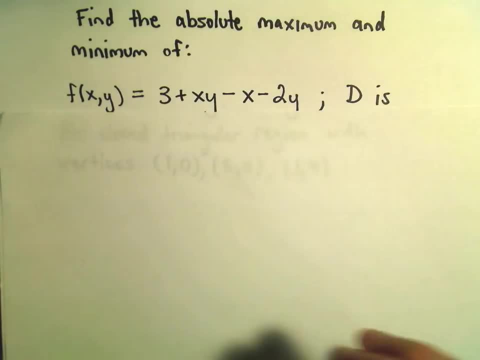 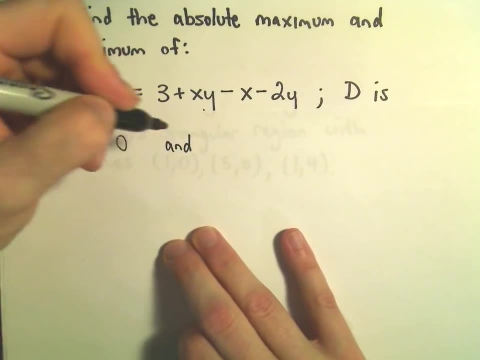 So, all right, a couple things we're going to have to do. We have to find, We have to take the partial derivatives. So we'll have to take the partial with respect to x, set it equal to zero, And we'll also have to solve the partial with respect to y. 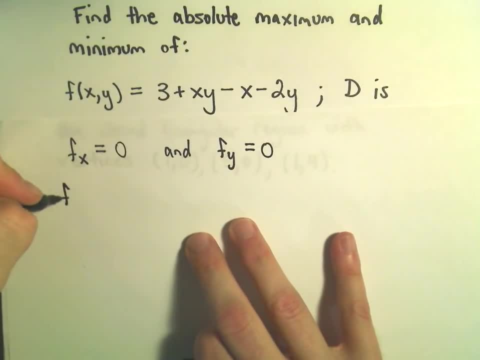 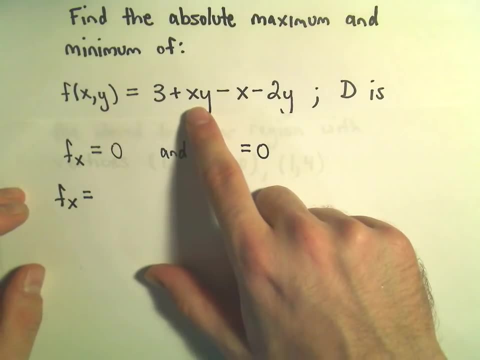 We'll set that equal to zero. Okay, so the first thing I'm going to do is take the partial derivative with respect to x. So let's see, 3 is just a constant, so that goes away. The derivative of x times y. 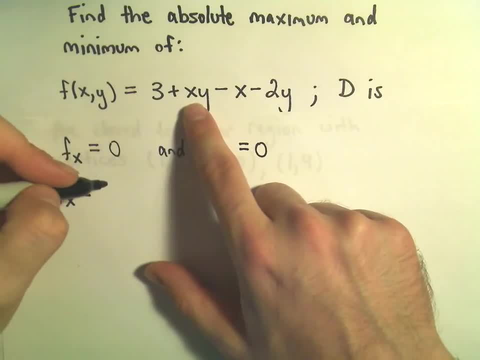 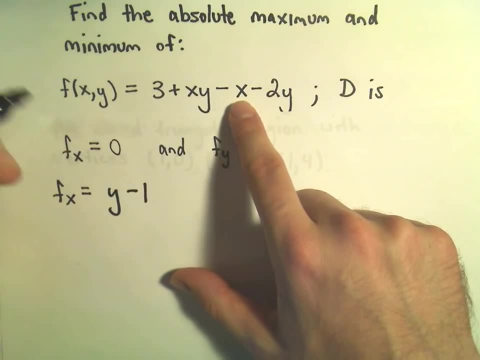 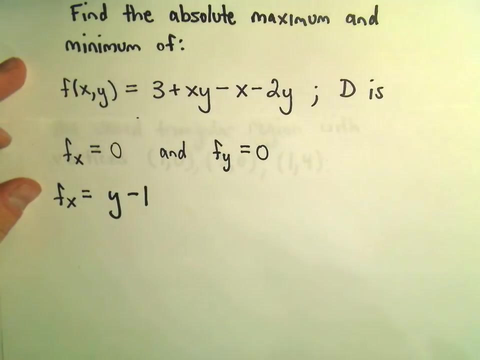 Okay, so we're treating y like a constant, So our derivative would simply be y. If we take the derivative of negative x, that'll leave us with negative 1.. And if we take the derivative of the negative 2y term- again, since we're treating y like a constant, that will simply go away. 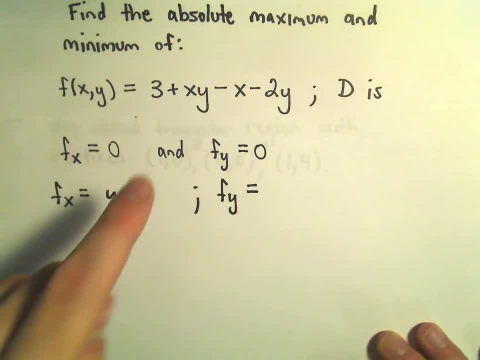 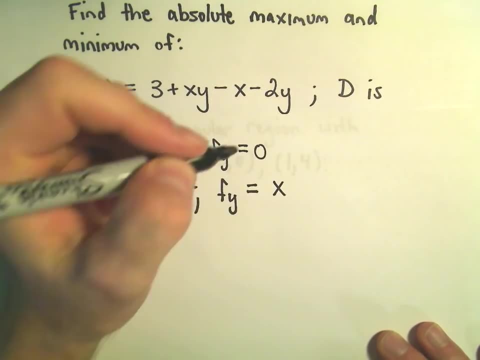 Likewise we have to take the partial derivative with respect to y. So again 3 is a constant, Then it goes away, y's now our variable. x is like a constant. So we'll just get x when we take the derivative of xy. 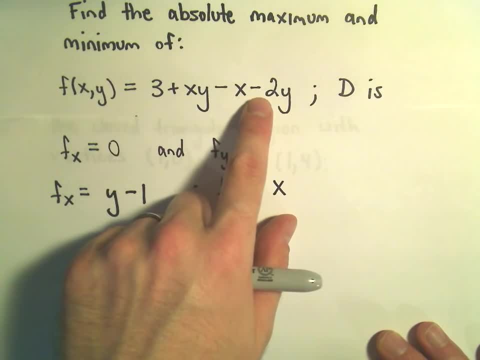 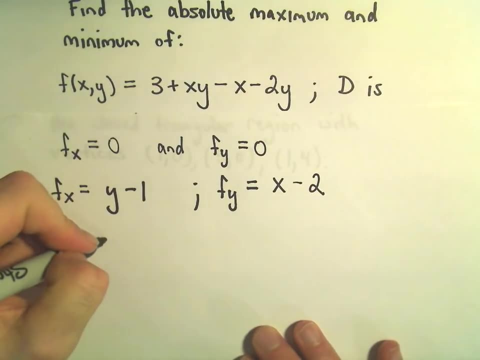 The negative x will simply go away, And when we take the derivative of negative 2y with respect to y, we'll simply get negative 2.. All right, so this isn't too bad. We have to set each one of these equal to zero. 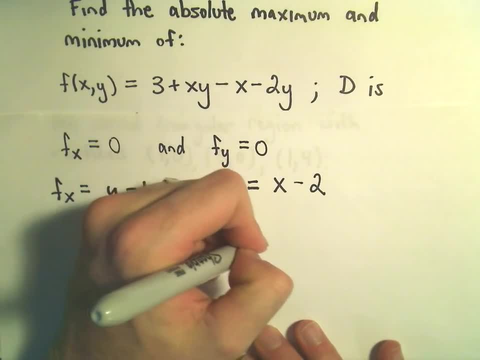 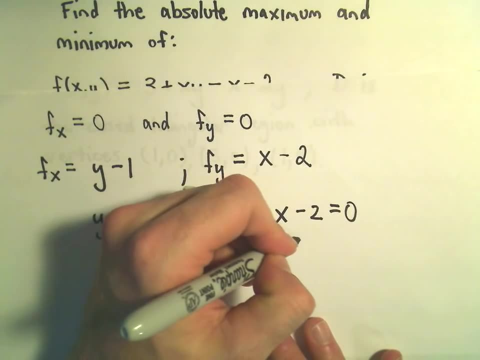 And we have to solve Whoops. I almost wrote another y, So we'll have to take x minus 2 and set that equal to zero. So obviously Not too bad equations here. x equals 2.. Doesn't get much better than this. 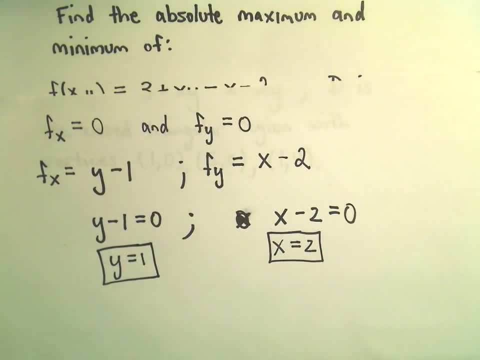 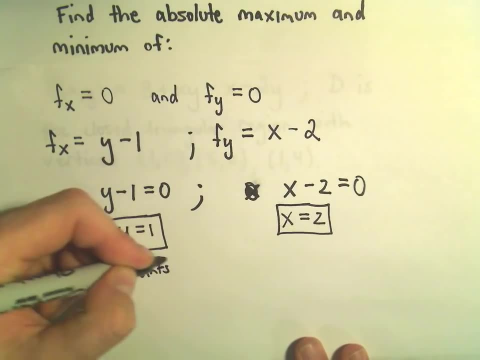 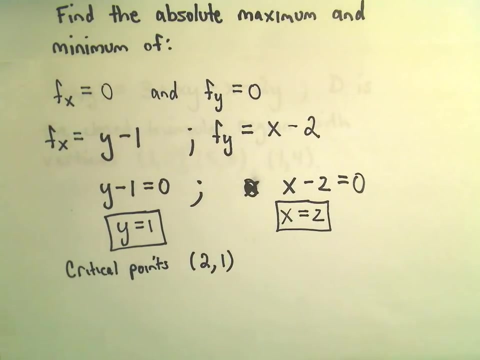 y equals 1.. So okay, so one of our critical points. it says it's going to be a 2, 1.. So we still have to kind of make sure you know that this critical point is within our boundary. 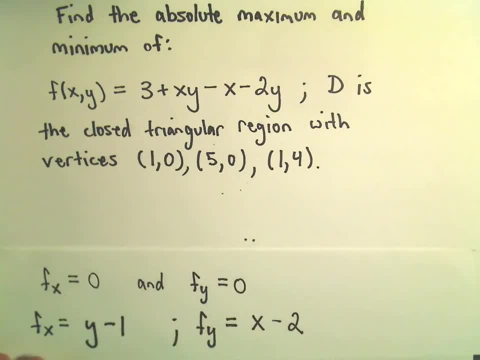 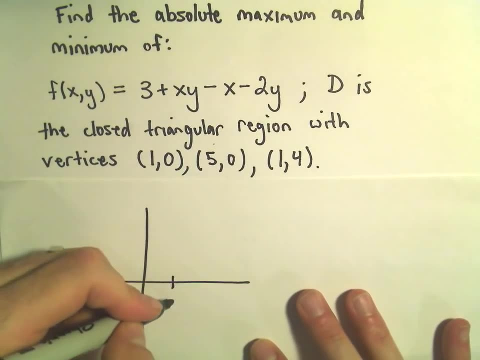 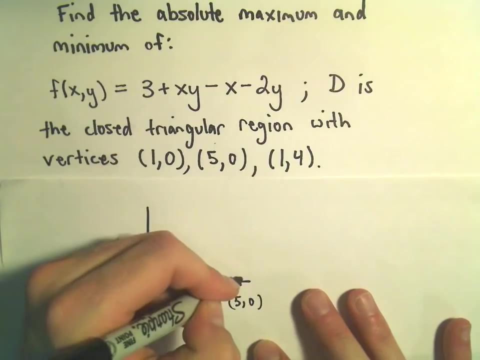 Because otherwise we won't even use it. So let's go back for a second and think about our boundary here. So we've got, We've got this triangular region. So 1, 0, that would be right there. 5, 0 would be right there. 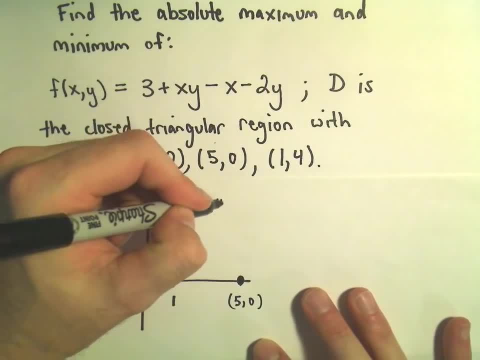 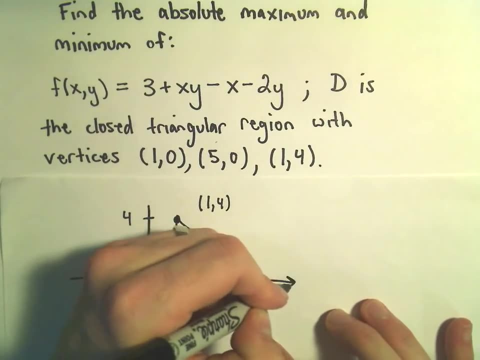 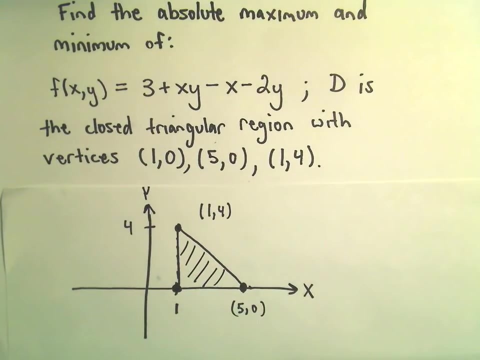 1, 4, that'll be up there. So we've got our little triangular region that we're talking about. So we're trying to maximize our function over this region, Okay, so certainly we found our critical point To be 2, 1.. 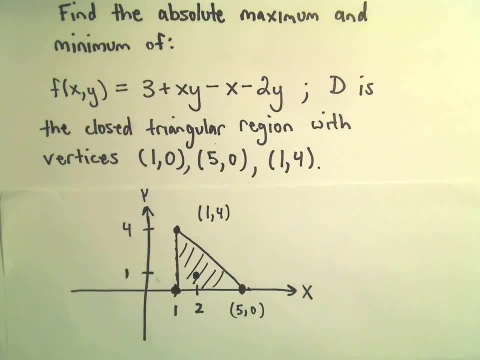 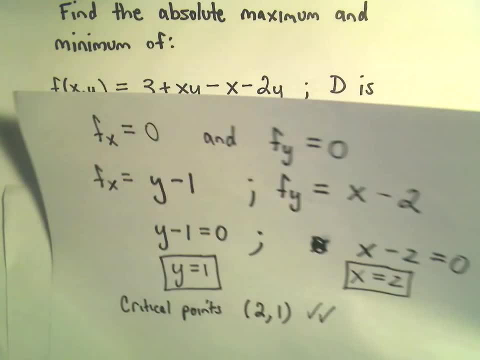 So certainly 2, 1 would definitely fall in that interval. So we will in fact evaluate our function at this critical point: 2, 1.. Okay, so now kind of the tricky part is we also have to evaluate this function on the boundaries. 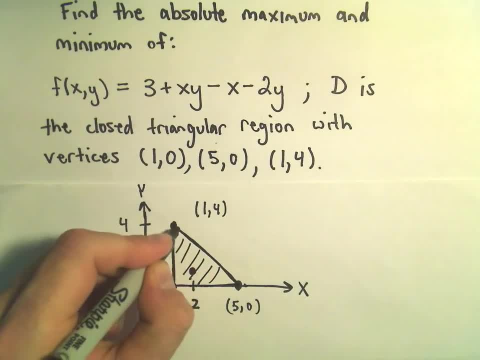 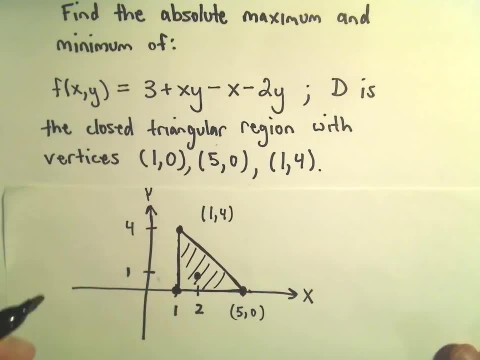 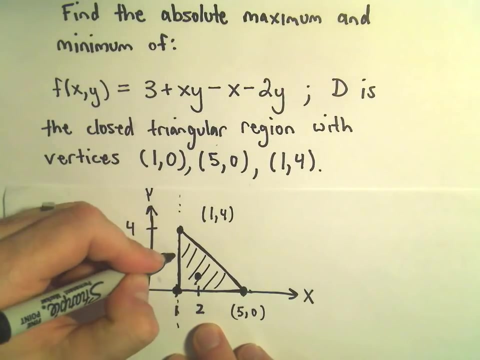 Okay, so this will kind of be the slightly longer part, So I think I'm going to break this up here into two parts. The first thing I'm going to do is find equations for all these. So you know, to find the equation of this line that goes through 1 and 4, well, that's easy enough. 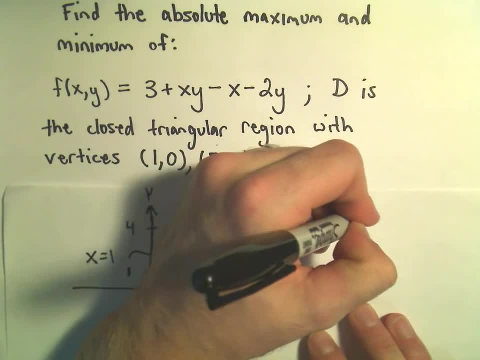 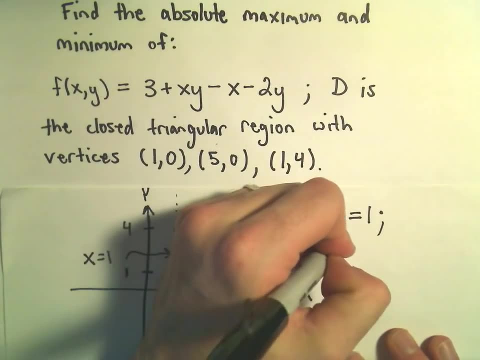 That's just going to be the line: x equals 1.. So that's going to be one of our boundaries. Let's see another boundary at the bottom. that's just going to be y equals 0.. So that's not bad. 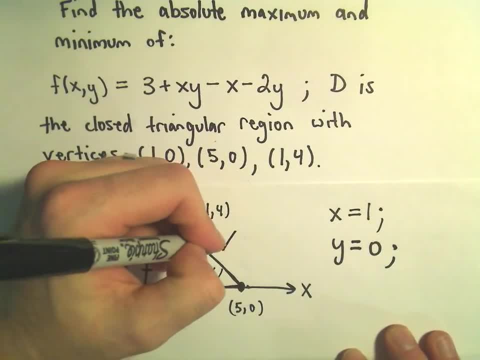 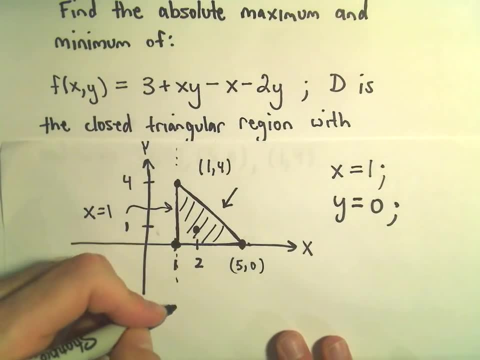 That's going to be another one of our boundaries. And then we also have to find an equation for this line. Well, however you want to do it, I'm just going to use point-slope form. So, if we take y minus, I'm going to use this point on the line. 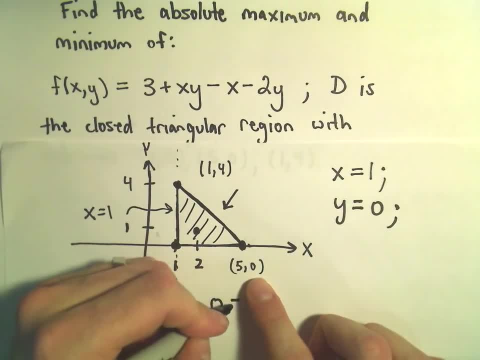 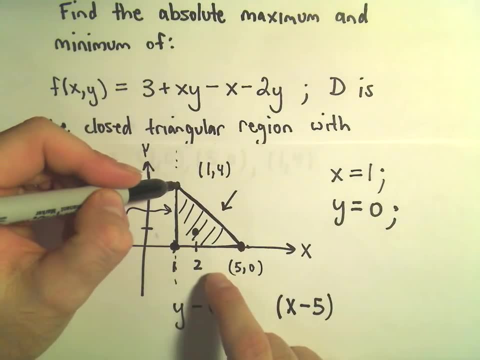 So I'm trying to just find the equation of this line. I'll use y minus 0. We'll figure out the slope x minus 5.. Well, let's see the slope. if we go from 1, 4 to 5, 0, we would go down by 4.. 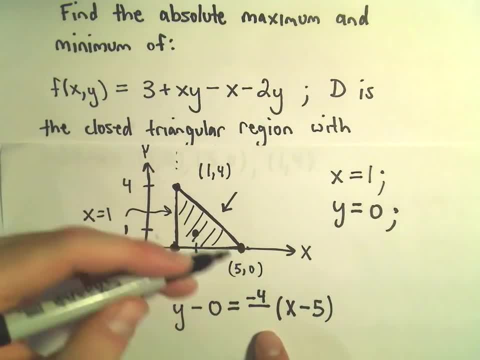 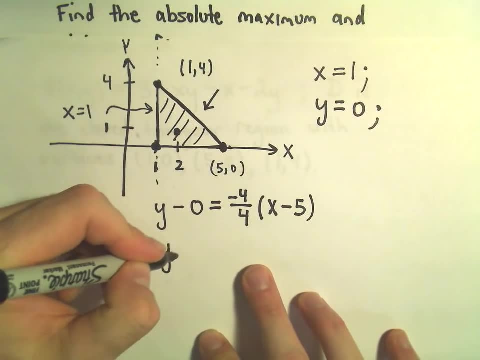 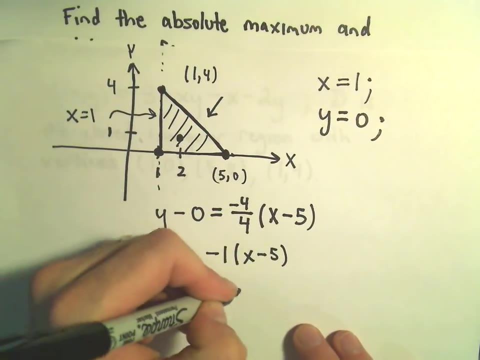 So change in y is just negative 4.. And then, if we go from 1 to 5, that'll be a change in x equal to 4.. So it looks like we're simply going to get the equation: y equals negative 1 times x minus 5, or, equivalently, y equals negative x plus 5.. 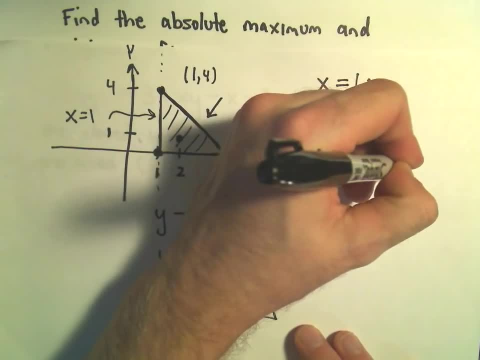 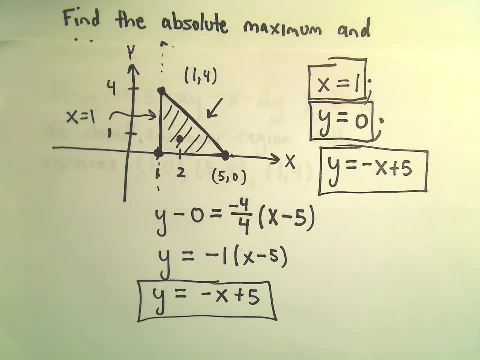 So that's going to be another one of our boundaries, And now we'll kind of begin this process. Okay, so plugging our critical point, this critical point 2, 1, back into the function. that's easy enough. You know, we'll do that here in a second. 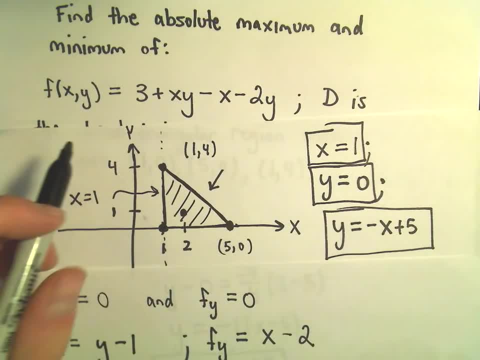 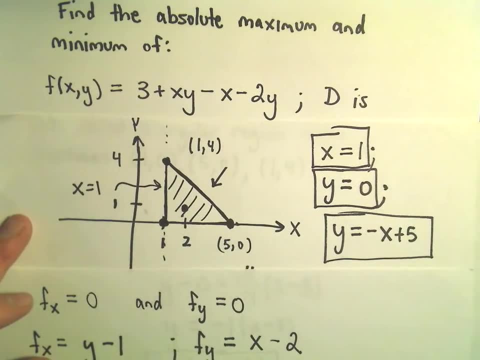 We'll plug 2 in for x and 1 in for y. Now we're going to do this function. We have to maximize this original function over each one of these boundaries, And that'll be the slightly more tedious part. So I think I'm going to do that in a separate video. 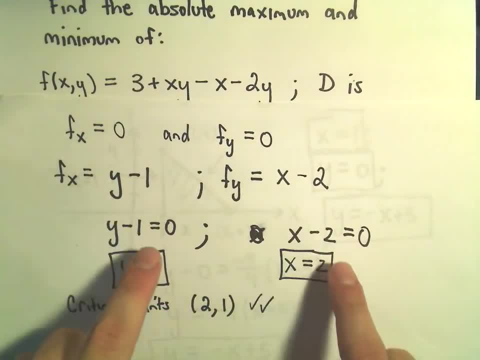 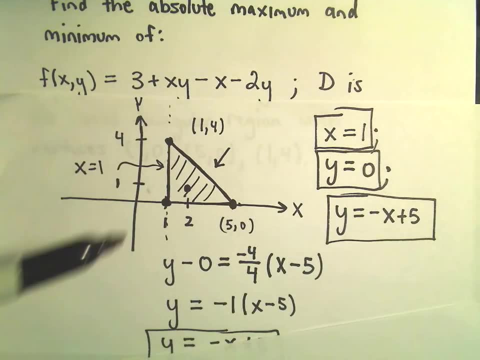 But again, this is kind of the first step. You just have to take the partial derivatives, set them equal to 0, solve, You know. obviously, again, these are pretty easy partial derivatives, nothing too crazy there. Check that your critical point is in the boundary that you're given, the region that you're given. excuse me, 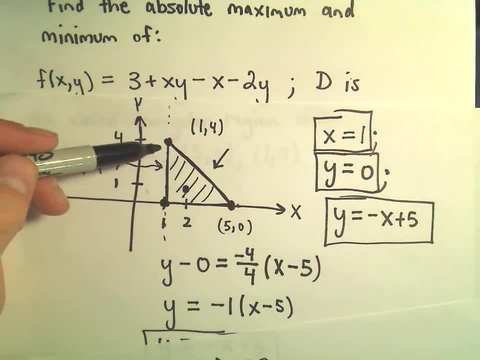 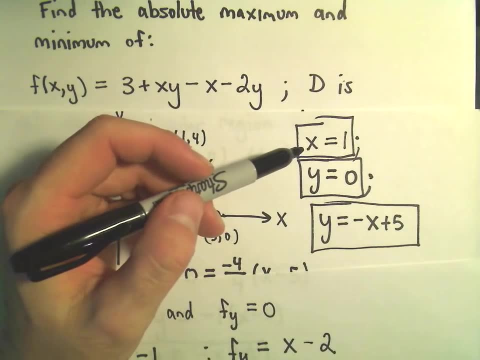 Find equations for all the boundary curves, Whatever you have, Whatever they may be. Hopefully you'll get kind of a simple boundary like I have here. It's just lines, But now the tricky part, or kind of the not even tricky, but it's just going to take a few minutes. 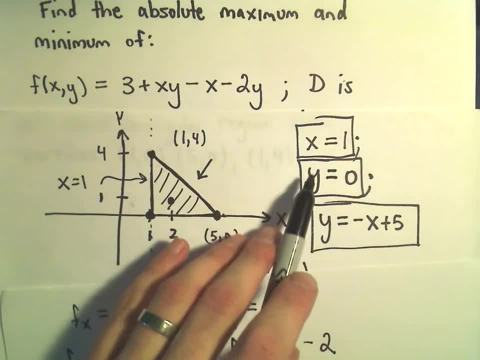 Again. now we're just going to have to plug. we're going to have to somehow evaluate our function at these boundaries. So, alright, stay tuned. We'll do that in another video. 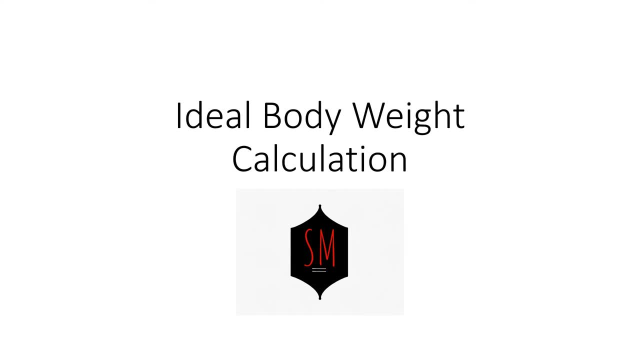 All right, we've got a short and sweet video today going over ideal body weight calculation. The ideal body weight calculation is indicated in the ICU when we start working with ventilators, and we can talk about that later. but this video is just for you to understand the ideal body weight calculations. So we're going to- for males, we're going to take the 50 plus 2.3 times the height and 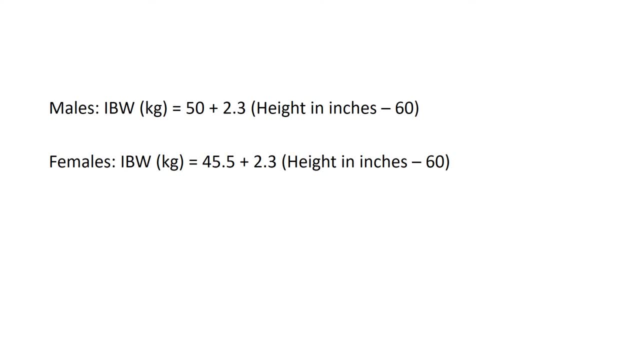 inches minus 60, and for women you just do 45.5.. So these are pretty easy formulas to memorize and it would behoove you prior to your ICU rotation to to get these down. So let's do a quick practice problem: What is the ideal body weight of a 5 foot 10 inch male? 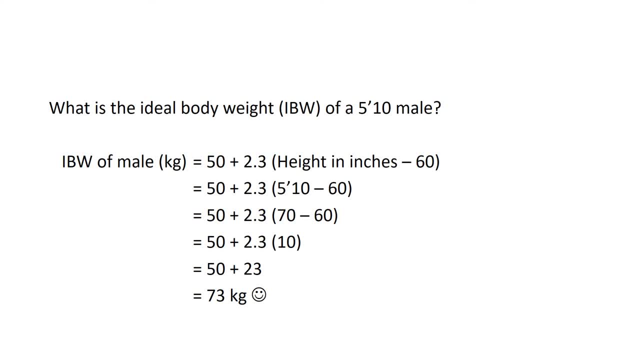 We'll fall back on our formula. We'll take the height in inches, 5 foot 10, so that's a 70 inches from 60 from 70 is 10 times 2.3 is 20.3 plus 50. that gets us 73 kilograms.